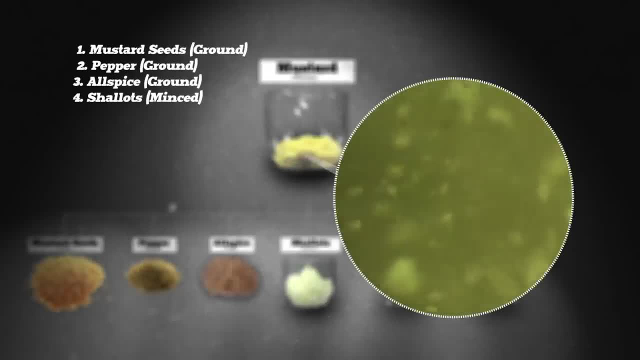 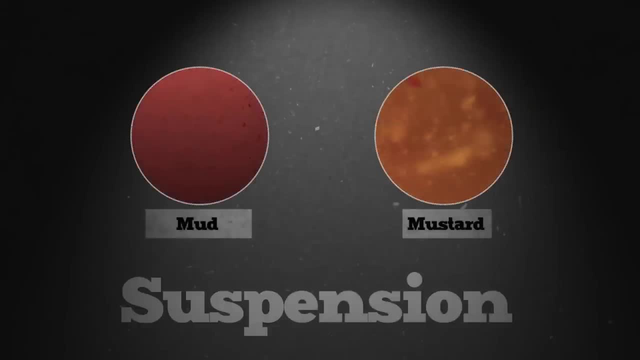 of little particles like mustard, seeds, pepper, allspice and minced shallots, all floating around in a liquid, In this case vinegar and water. This is called a suspension, because you've got particles of one thing suspended in another. Now on the other end of the spectrum is a solution? The 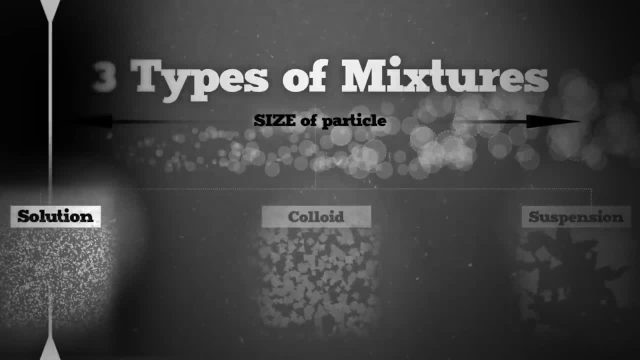 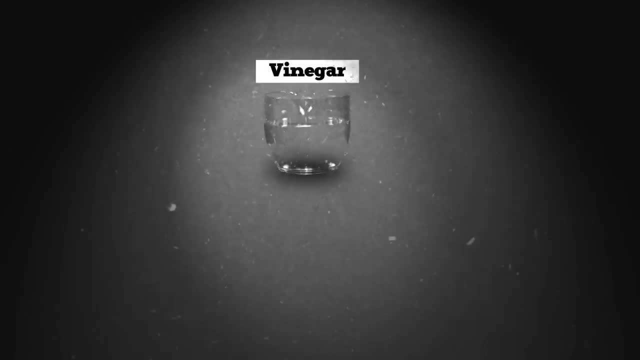 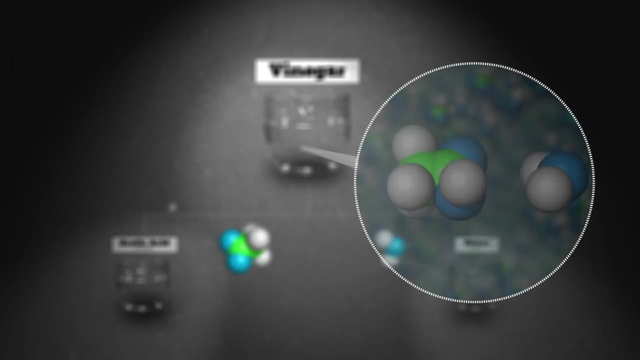 particles in this mixture are so small they are the actual molecules. A solution is sort of like a suspension of molecules, where one type of molecule is blended or dissolved with another. Vinegar is blended with molecules of water. The chemical properties of the molecules haven't changed. they're. 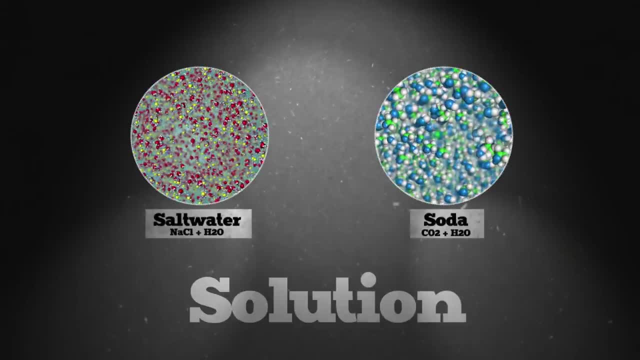 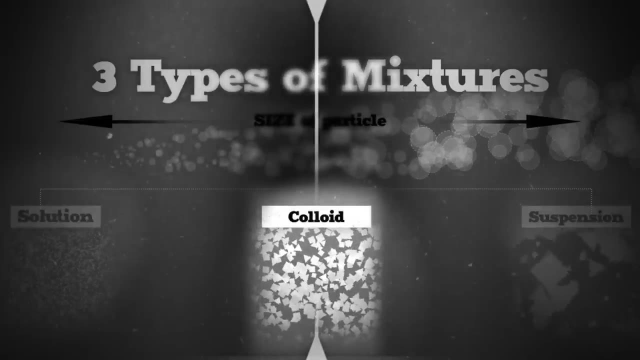 just evenly mixed together. now, Salt water and carbonated soda are both examples of solutions where other molecules are dissolved in water. The last type of mixture is called a colloid, which is somewhere between a suspension and a solution. It's when you take two materials that don't dissolve. 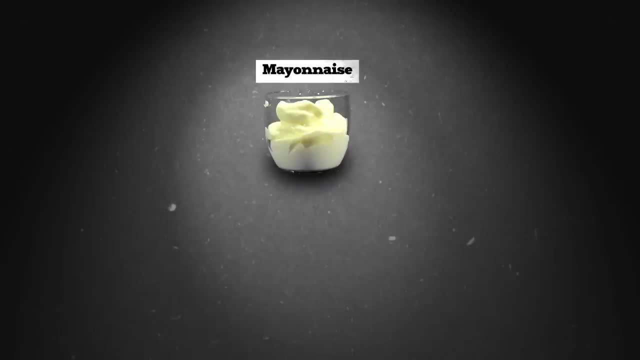 and you make the particles so small that they can't separate. Mayo is what happens when you take oil and water which don't mix and you bind them together, usually with the help of another substance called an amalgam. In the case of mayo, it's emulsifier. In the case of mayo, it's lecithin found in eggs. And now you're 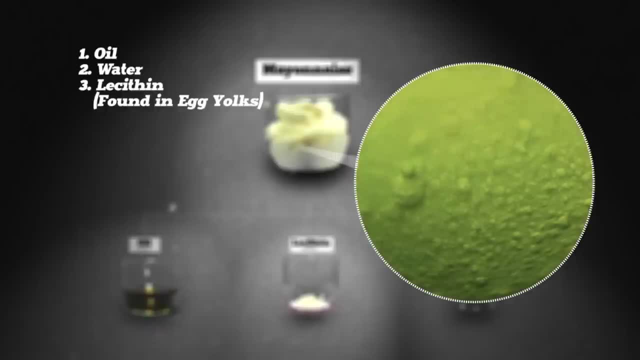 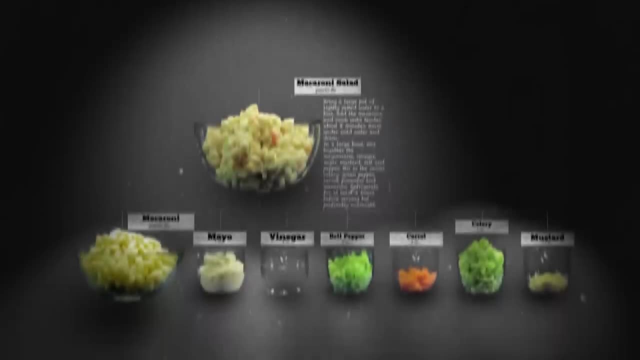 left with really small globs of oil hanging out with really small droplets of water. Whipped cream, hairspray, styrofoam and jello are all other examples of colloids. So let's get back to macaroni. 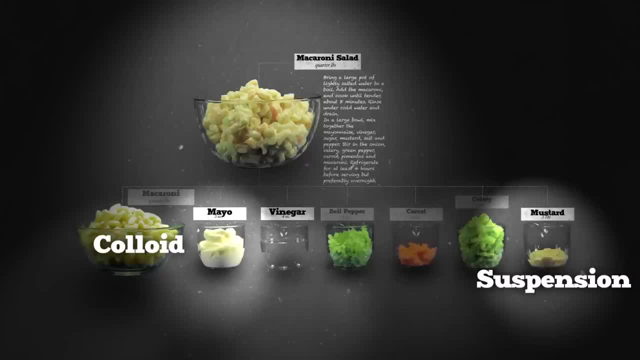 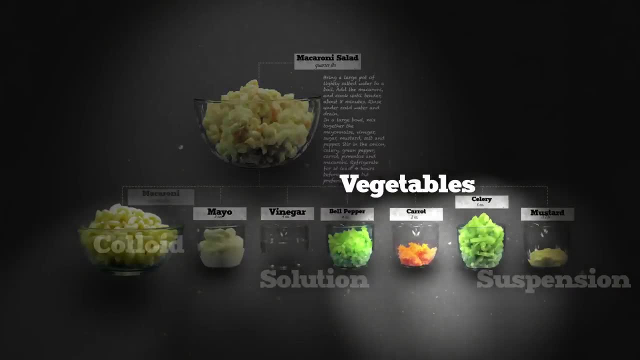 salad. You've got colloids like mayo, suspensions like mustard and solutions like vinegar, But you've also got celery, shallots and all other vegetable chunks that are also part of the salad. These aren't mixtures really, but we can break them up, just like a TV can be broken up, and 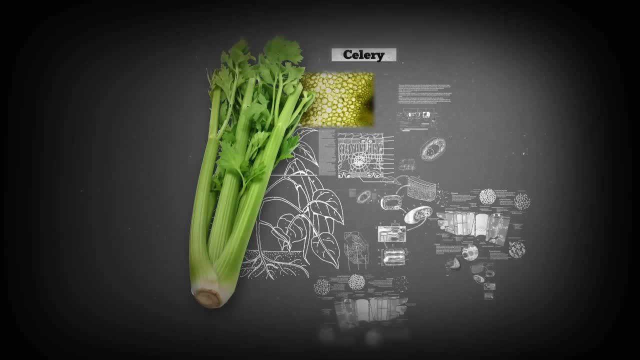 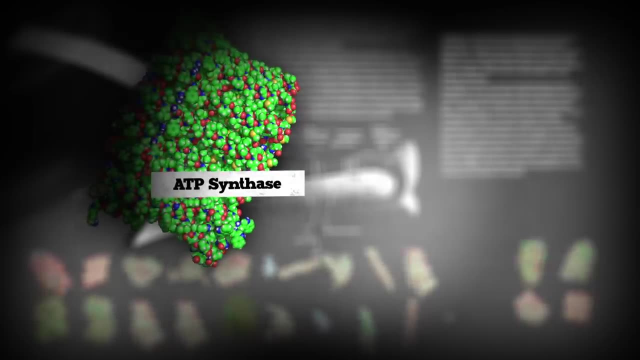 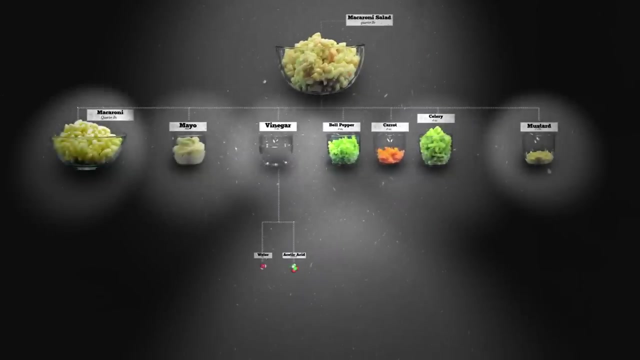 into smaller and smaller complex component parts. In the case of vegetables, if you keep breaking things up, it will eventually end with thousands of complex organic molecules, Things like ATP synthase and RNA transcriptase and water. So now, once we've unblended all the solutions, 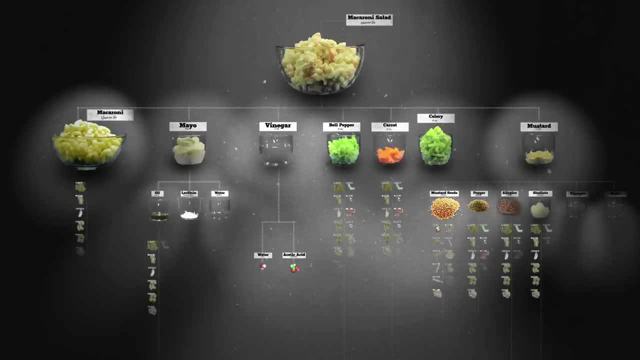 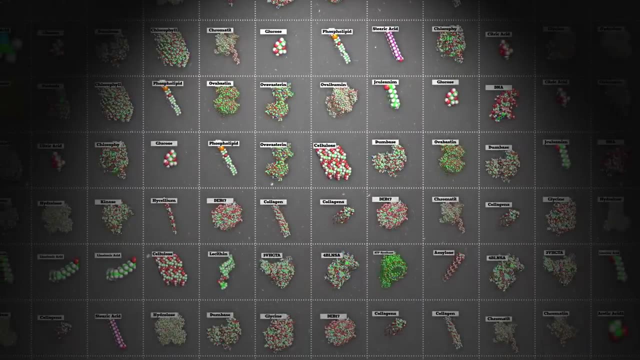 unmixed all the colloids, separated all the suspensions and taken apart all of our vegetables, we've reached the end of what we can unmix physically. What we're left with is a whole bunch of molecules. These molecules remain chemically the same whether they are by themselves or thrown together.